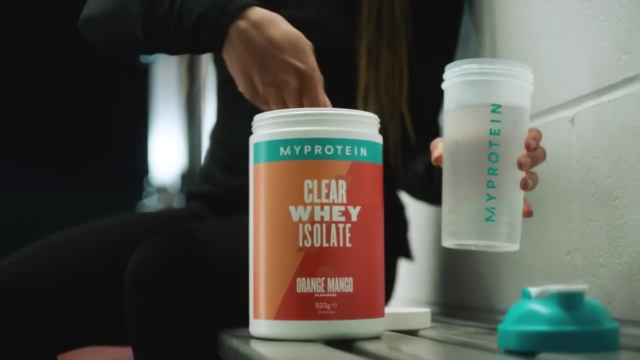 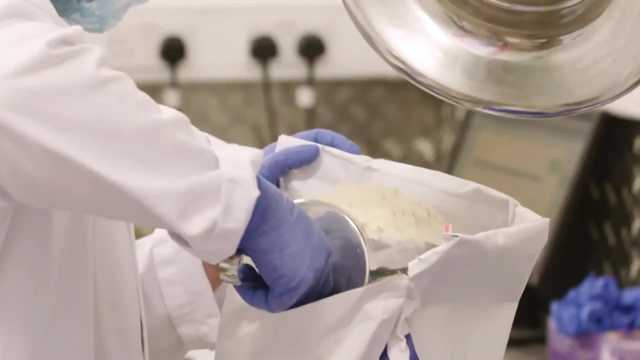 If it's just a solid, reliable, no-frills product you're after, this could be the best protein powder for you. MyProtein prides itself on providing an all-round value-for-money product. It's ranked Grade A by independent tester Labdor for both quality and value. 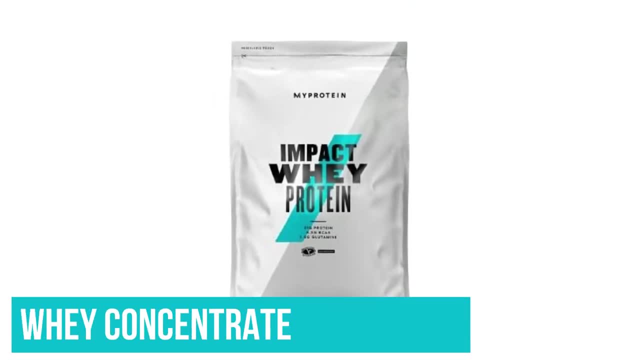 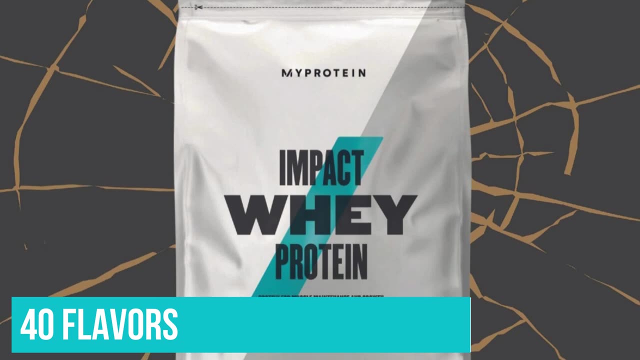 The protein comes from whey concentrate, which some people find causes bloating. There are few ingredients, although some of the flavour options include artificial flavours. It comes in more than 40 flavours and a range of sizes. We found the 250g bag really useful. 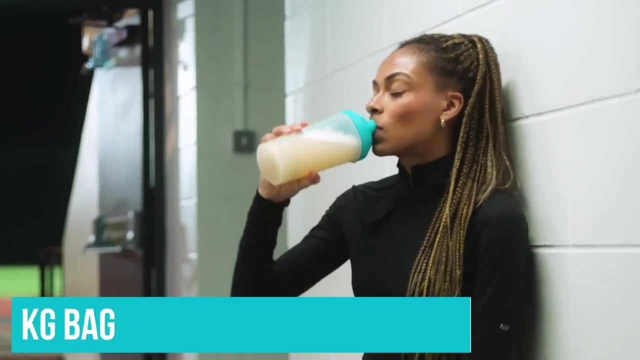 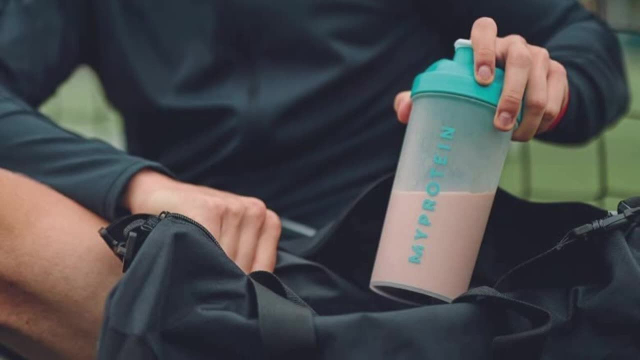 for a weekend away or bringing into the office, but you can also purchase a 5kg bag to store at home. If you're bewildered by the choice, consider buying the sample pack, which contains up to 8 flavours to try before you commit to a larger size. 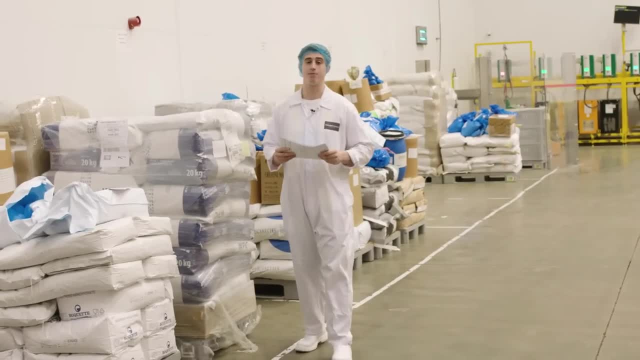 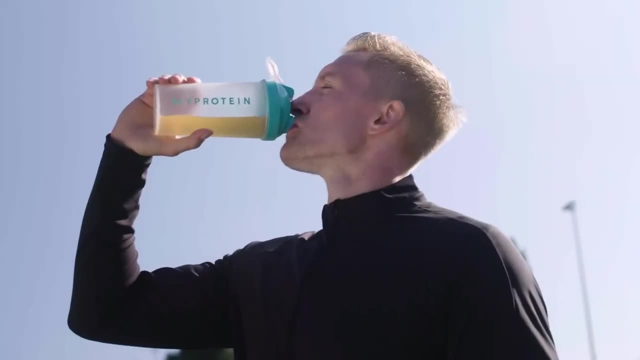 We tried the chocolate smooth, which worked well when stirred into porridge, although if you're after more of an intense chocolate taste, the chocolate brownie may be more to your liking. We also liked the sticky toffee pudding flavour, whilst those who liked something a bit more. 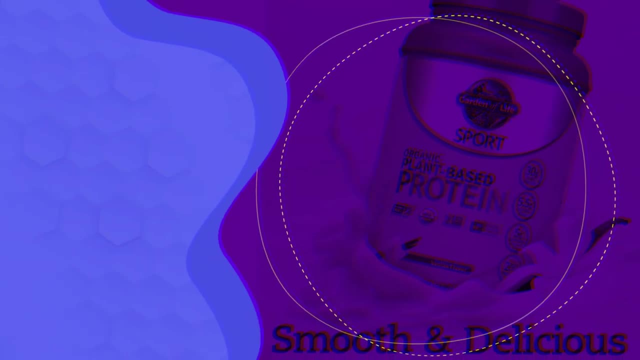 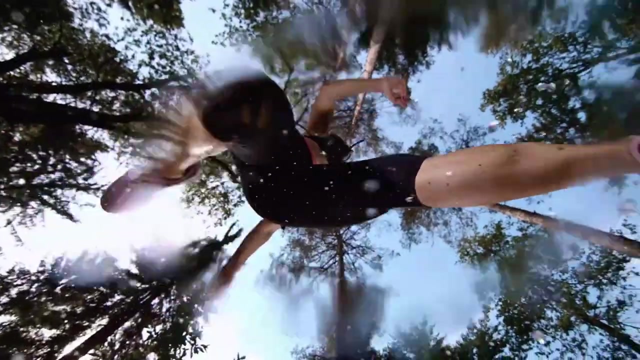 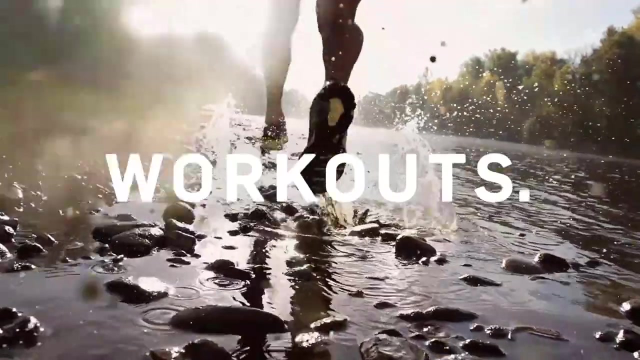 simple favoured: the vanilla and the strawberry. Number 4.. Garden of Life Sport Organic Plant-Based Protein Powder. If you're looking for a flavoured protein powder that doesn't overpower your beverage, Garden of Life's Sport Organic Plant-Based Protein Vanilla is a top choice. It lends a mildly sweet vanilla flavour to smoothies. 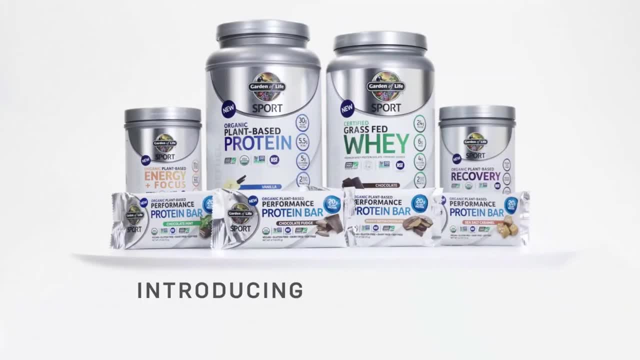 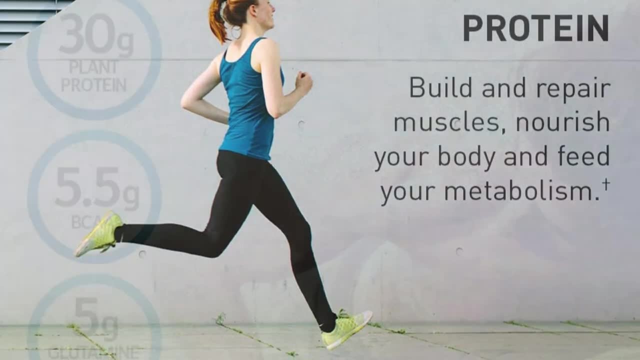 or other recipes, or can be enjoyed just mixed with your favourite milk or water. The protein comes from peas, navy beans, garbanzo beans, sprouted lentils and cranberry protein, and it's combined with vanilla, stevia and a little sea salt for flavour. It's also a great. 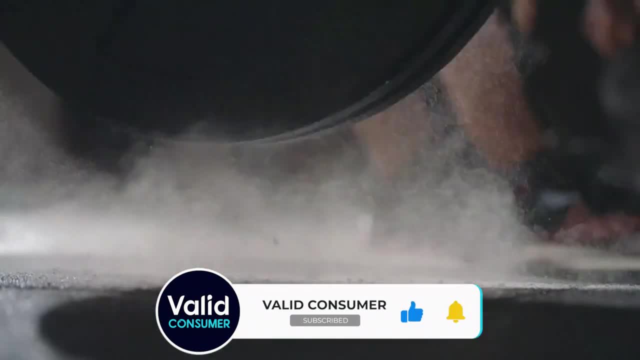 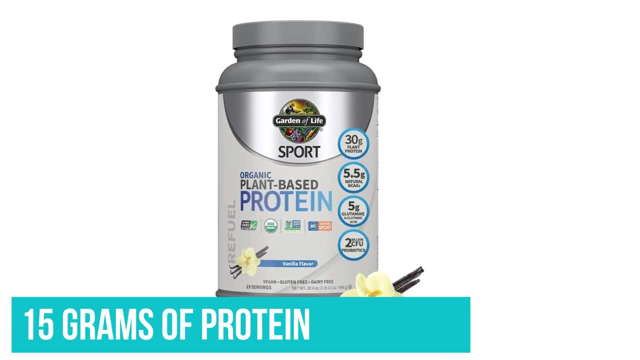 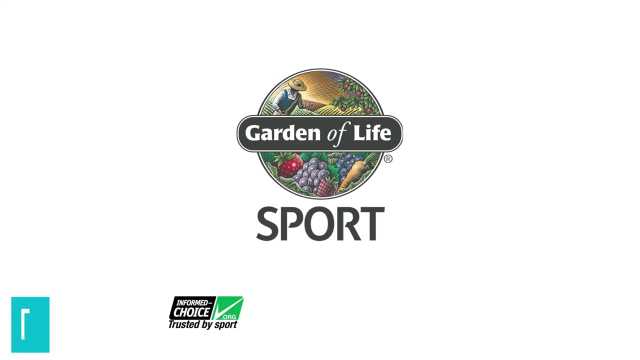 option for active people, as it contains a recovery fruit blend, including tart cherry, which may improve muscle recovery in both strength and endurance athletes. Just one scoop provides 15g of protein and 20% of your daily iron needs, plus several other vitamins and minerals which may be helpful for those on a plant-based diet. 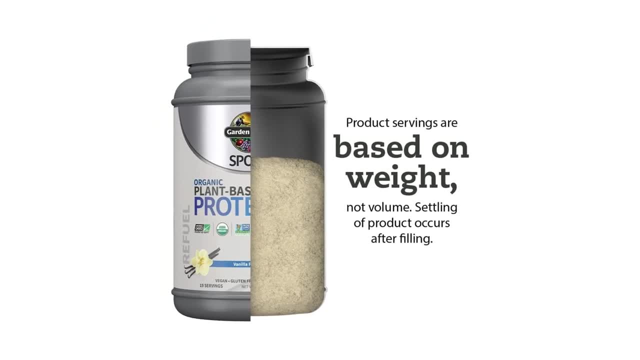 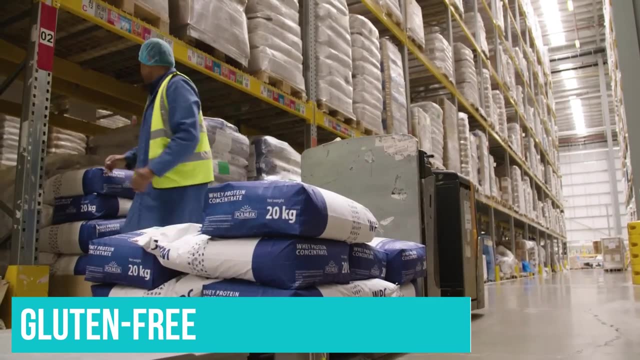 Garden of Life's Organic Plant-Based Protein Vanilla is approved by two of top third-party testing organisations: NSF Certified for Sport and Consumer Lab is gluten-free, vegan, non-GMO and kosher. It doesn't contain any of the top 9 allergens. 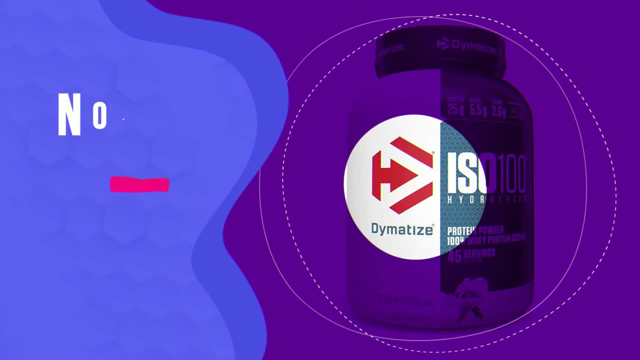 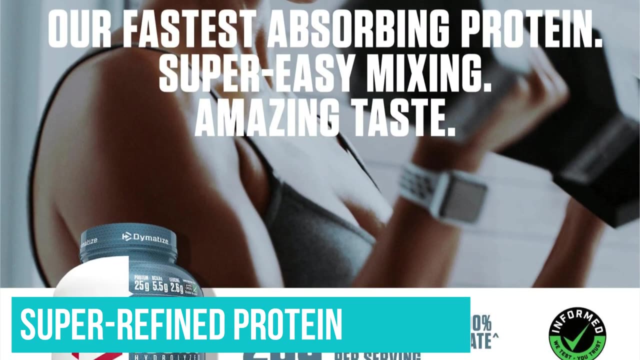 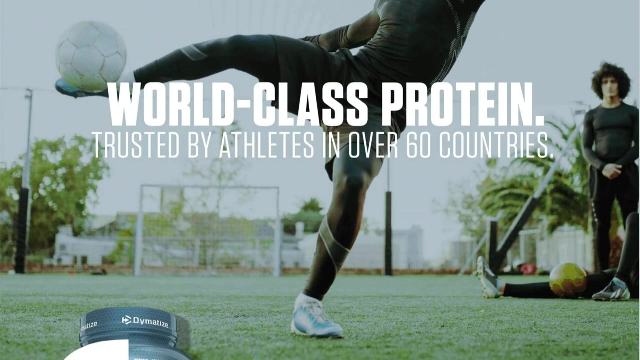 making it a good choice for anyone with food allergies. Number 3. Dymatise Nutrition ISO 100 A super-refined protein product. this is the best protein powder for anyone serious about building lean muscle. With the protein all coming from whey protein isolate, it's great for anyone. 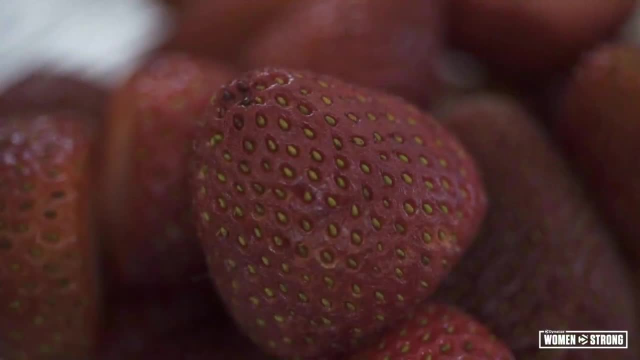 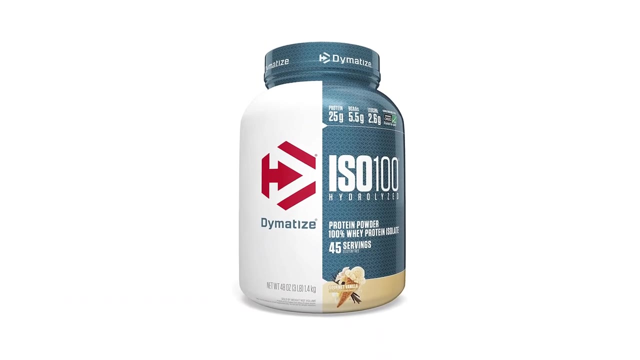 who struggles with weight concentrate and it's low in carbohydrates and calories. The inclusion of hydrolyzed whey protein isolate means you absorb the protein even more quickly. The flavour is good, without the temple-aching sweetness you get in some protein powders. 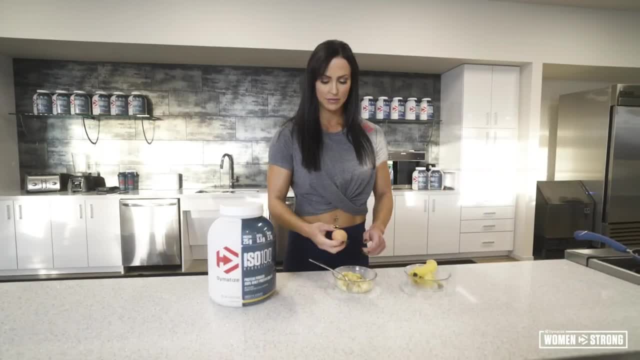 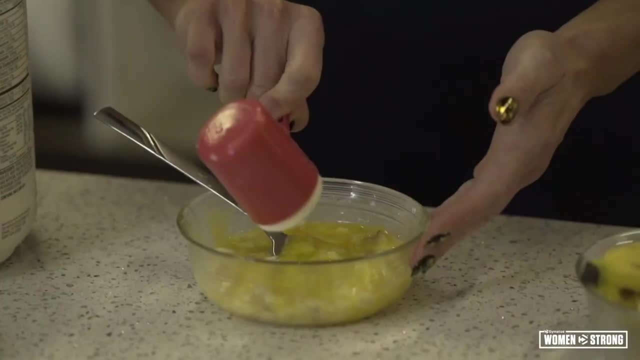 We tried the birthday cake flavour, which can be notoriously sweet, and even this was pleasantly tasty, but not overly synthetic. It mixes pretty easily too, although it's worth noting that, whilst some protein powders mimic the action of thickening agents when stirred into porridge, we found the Dymatise actually. 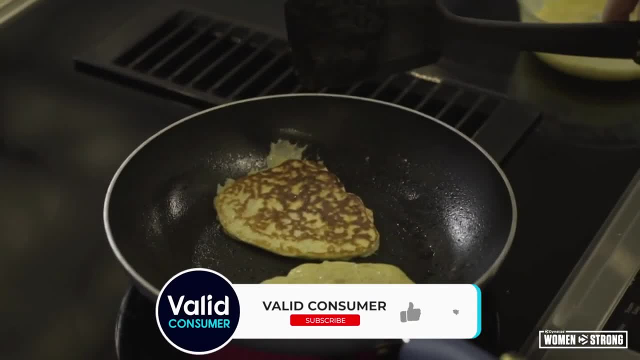 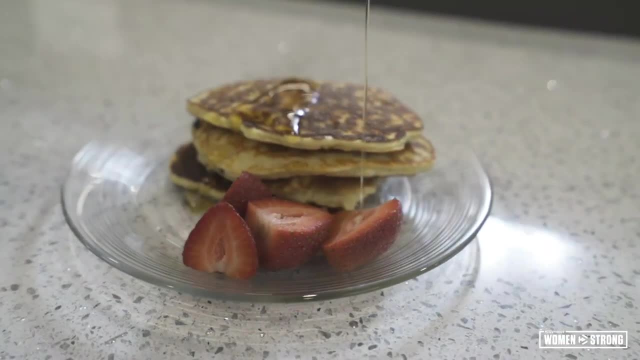 had the opposite effect and made the porridge slightly runnier. A draw is that there's a large variety of flavours to choose from, though it's a pity you can't buy it in sample sizes to try before committing to a large tub. The tub sizes are 900g or 2,200g, which is a lot of powder to 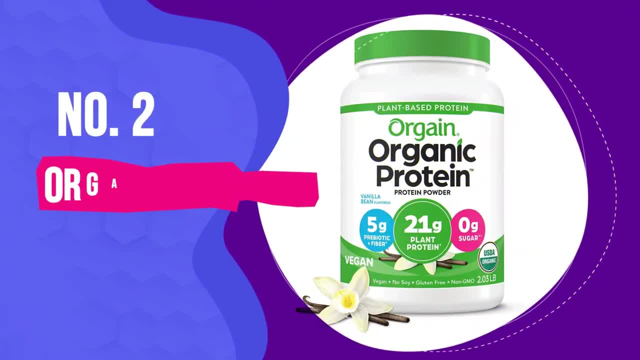 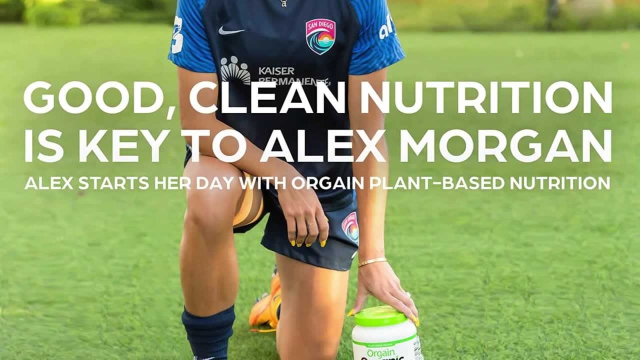 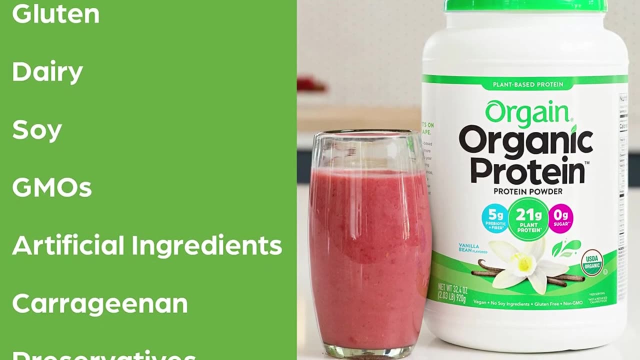 get through if you don't like the flavour. Number 2. Orgain Organic Protein. Some protein powders can contain processed ingredients that you might not recognise. However, if you're keen on finding a protein powder filled with natural ingredients, the Orgain Organic Protein Powder might just be. 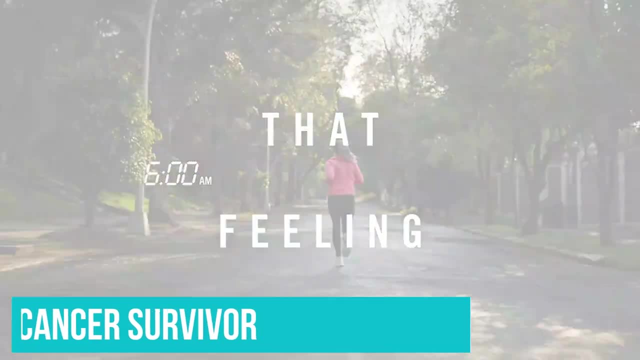 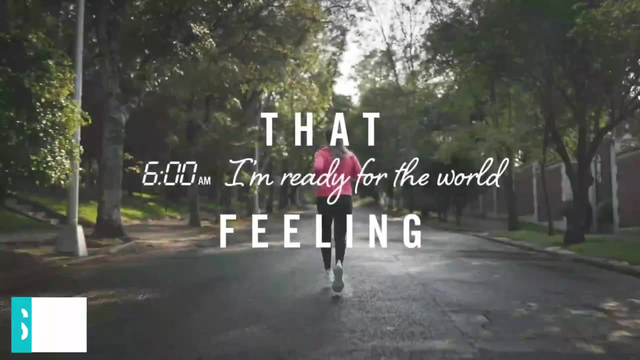 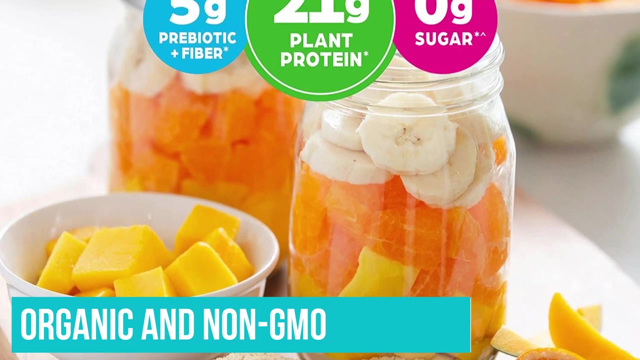 the one for you. Founded by a cancer survivor and integrative specialist who wanted to create a product with natural food-based ingredients, Orgain makes products with ingredients that, whilst perhaps not exactly familiar, are at least recognisable foodstuffs, and the powder is certified organic and non-GMO. Be aware that the calorie count is 150 per serving. 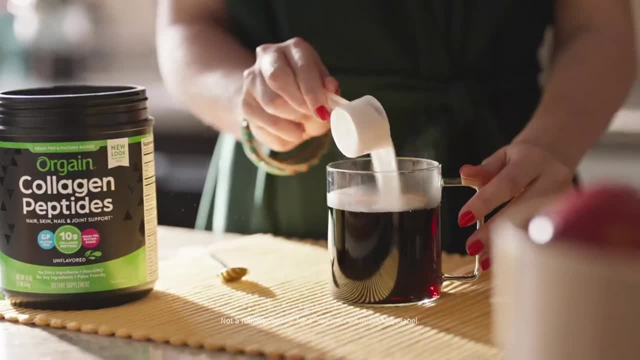 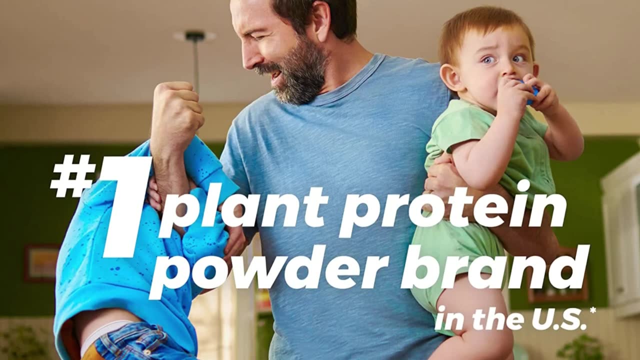 which is a little higher than most non-mass gainer powders, and the carbohydrate count is 15g, so it's not low carb. It contains sea salt, so if you're trying to keep your sodium levels down, this may not be for you. 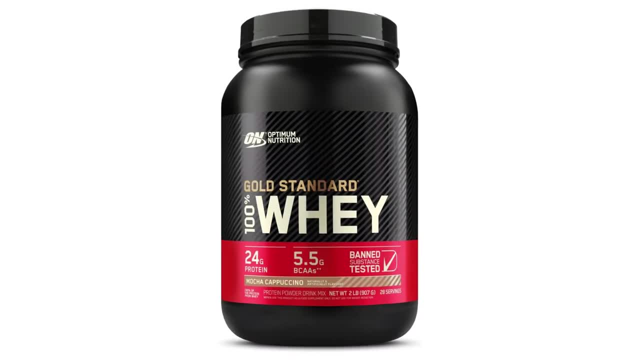 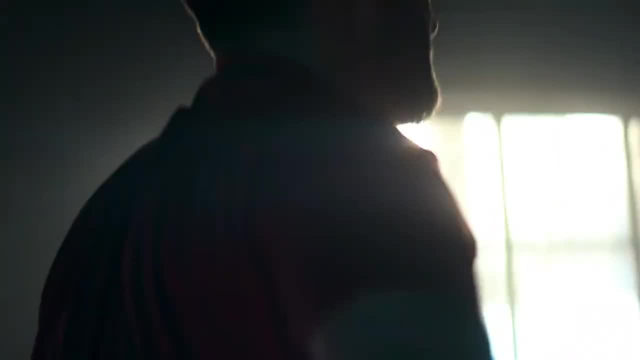 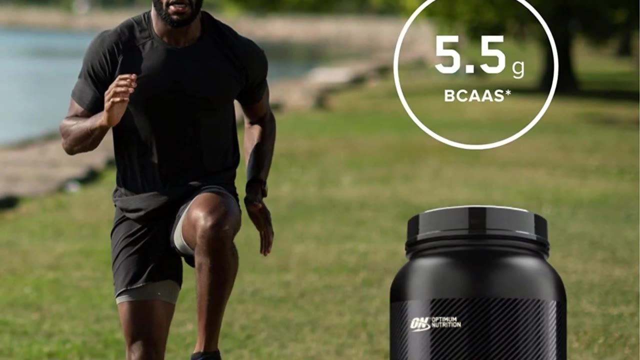 Number 1. Gold Standard Whey Protein. Many protein powders come complete with a range of flavours, some more palatable than others. However, if you want the flexibility to add your own flavours or you dislike the sweetness found in flavoured whey products, this is a great choice. It's not entirely flavour-free, but the